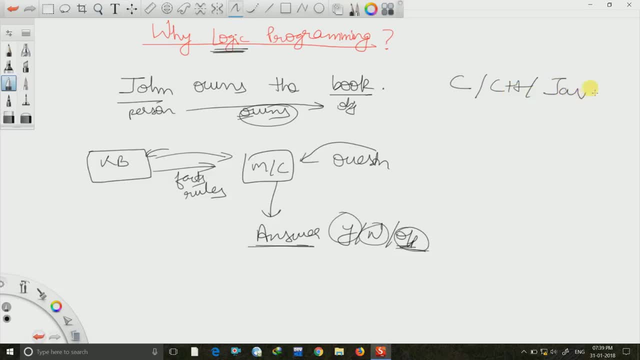 language. So C or C plus plus or Java. we don't use any knowledge base, you just have to include the libraries. First you have to include, include all the libraries, then you start your main function And then you declare some variable, suppose int a and something like that, And then you write down. 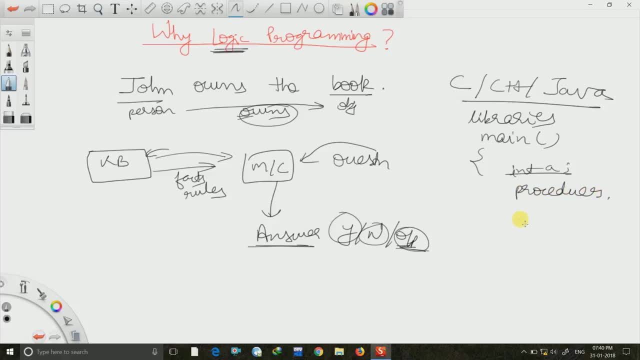 the procedures, how to calculate the output and then finally print the output. print the output and then return. Here's this was, this was the process in our conventional programming languages but, coming to logic programming languages, It is completely different And it has no relation with 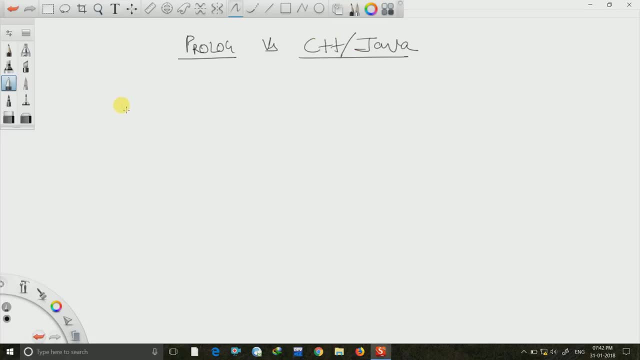 C or C plus plus or Java. If you are familiar with C plus plus or Java, then you must be familiar with object oriented programming And you know that in C plus plus and Java we use objects. So a problem is divided into different objects. 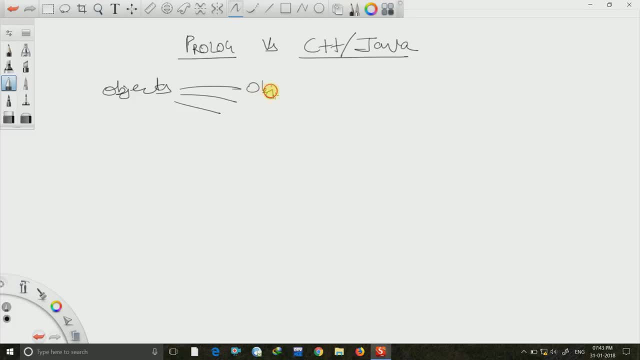 Ok, problem is divided into different objects and these objects are. these objects are combined. these objects are all combined for a particular answer, for a particular solution. okay, but in prologue we don't use object oriented programming. you might have heard me saying objects in prologue, so the objects in prologue are very different from that in C++ and Java. in C++. 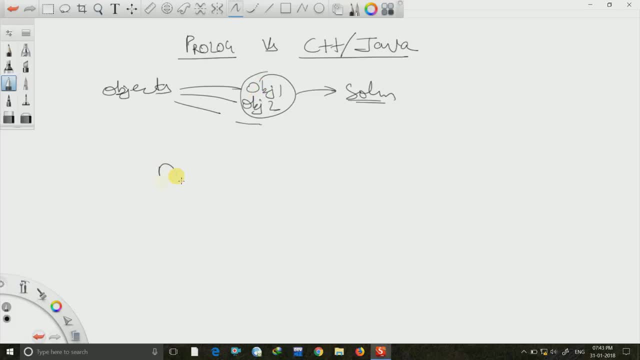 and Java. the object is a data structure. object is a data structure that can inherit fields and executable methods from a class hierarchy to which the object belongs. that means the classes. that means in the C++ or Java. if you create an object, then it can also inherit. 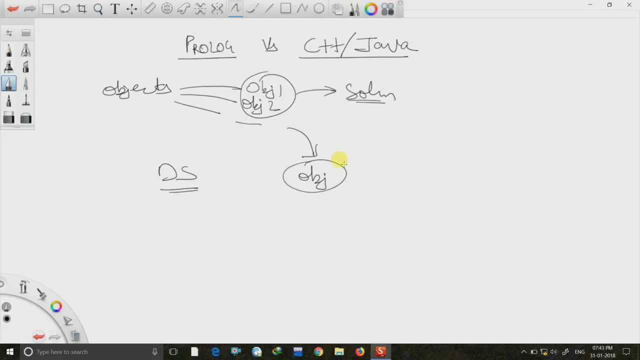 it can also inherit all the variables and the methods or functions from its upper class, that is, from its super class, if you are familiar with C++ or Java. If you are not familiar with C++ or Java or not familiar with the object oriented programming languages, then you should skip this part. now, in prologue, object is very different from. 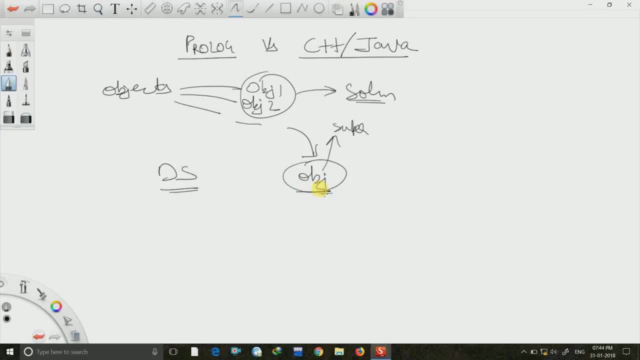 that in C++ and Java. I already told you the object in C++ and Java and in prologue the. I already gave you this example. John owns the book. okay, the book now here, the object is a data structure. So you can see that in prologue the objects are very close to the English meaning, while 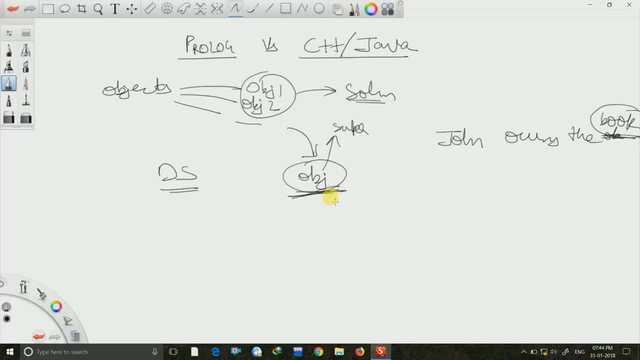 in C++ or Java. object is typically a data structure in prologue. the objects does not refer to a data structure that can inherit variables and methods from a class. it refers to things that we can represent using terms. so book is a thing which we can represent. 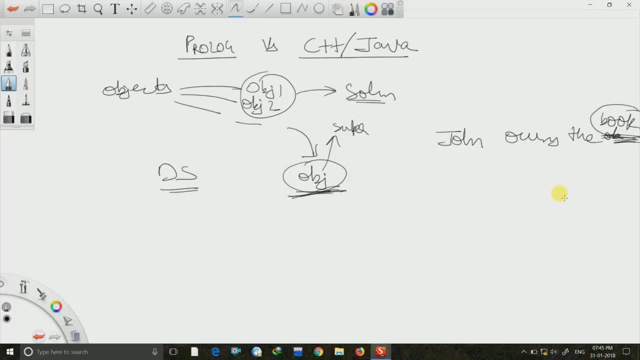 using terms, and hold on. I will tell you about terms, facts, knowledge base and all these things in our in our next tutorial. okay, so don't panic here. so, coming back to our question of why we should use logic programming, I can tell you that, in logic programming, if you are, if you are familiar, 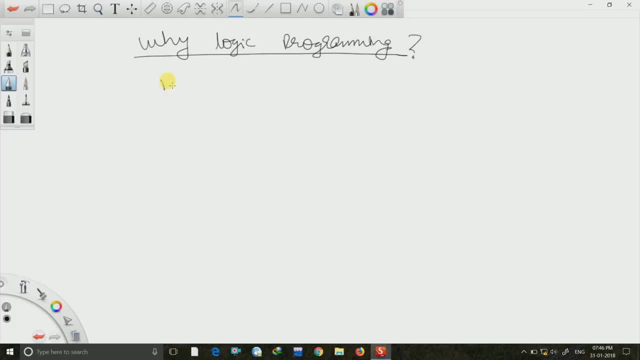 with the software development cycle, then you must be knowing that the maintenance of a software, maintenance of a software is the most costly part of the software development, because the software Development is not that difficult. but once the software has been developed, the maintenance of that software is the real challenge. okay, and the move most of the cost, around 60 percent. 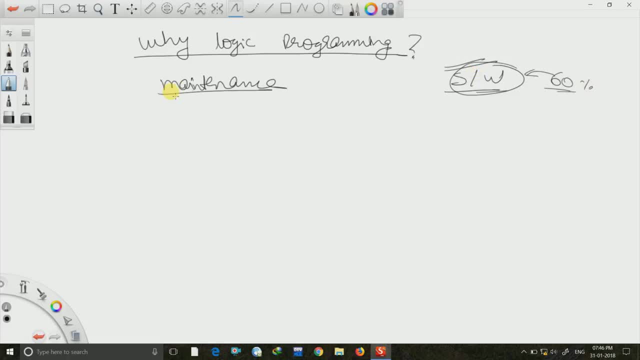 of the cost of the software is consumed in the maintenance process. okay, so this maintenance actually determines the final cost of the software. in prologue or in the logic programming example is prologue, the maintenance cost is drastically reduced, while in C++ or Java or other imperative or object-oriented languages, the cost is pretty high. so what is the reason? 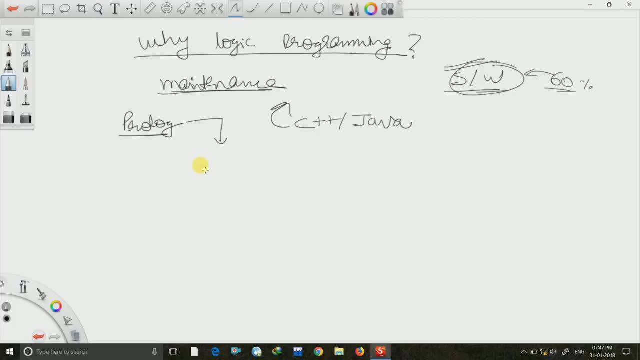 behind it in prologue. the readability of the code is very easy. readability of the code is very easy. so if you have, suppose, if a person A has developed a software, so person B can easily read that software, understand it very easily, and then he can modify a particular